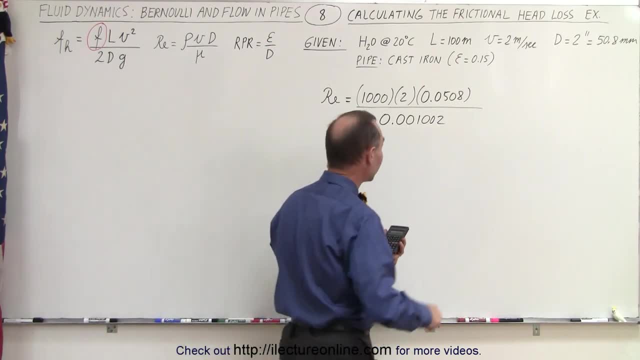 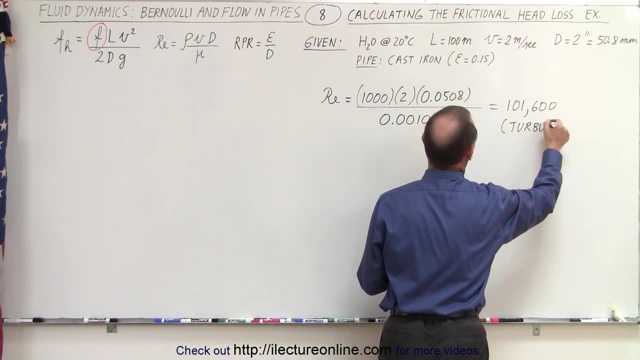 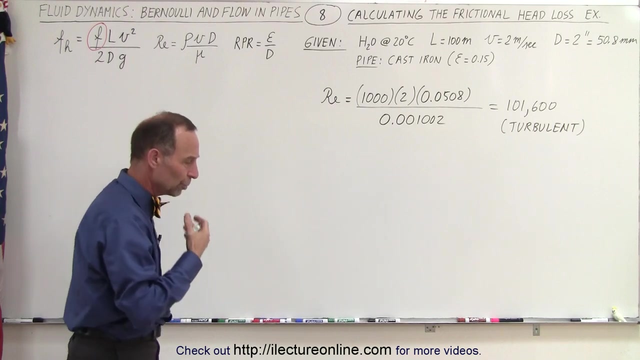 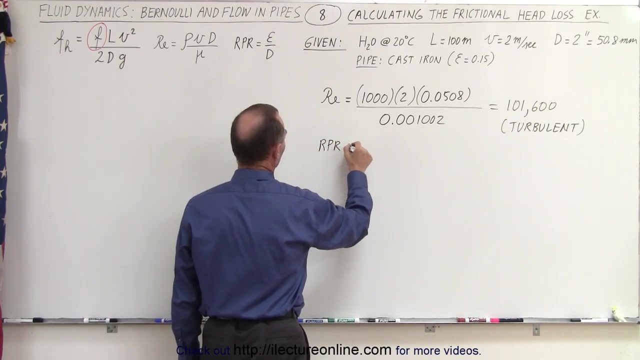 Equals and that's a pretty big Reynolds number, 101,600- and so therefore we can say that is probably turbulent, Most likely. All right, next thing we need to do is going to use the Moody diagram. We're going to need to find the relative pipe roughness, So the RPR is going to be the 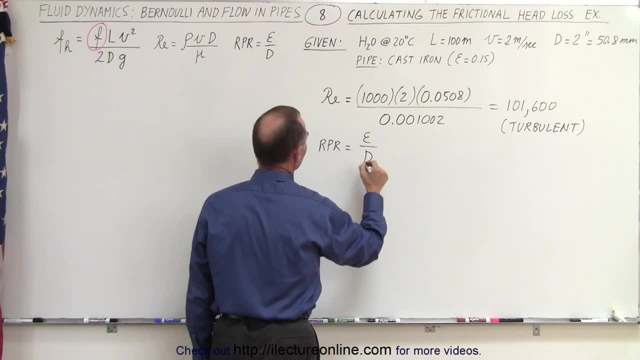 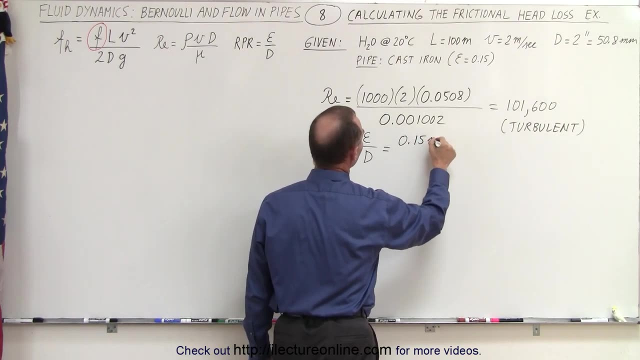 constant relative to the pipe. divided by the pipe diameter It's going to be in millimeters. So for cast iron that is 0.15 millimeters. and then we have to divide that by D and that would be in millimeters 50.8 millimeters. And so when we do that division, 0.15. 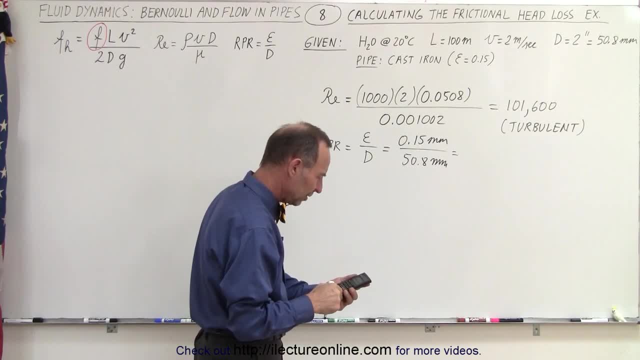 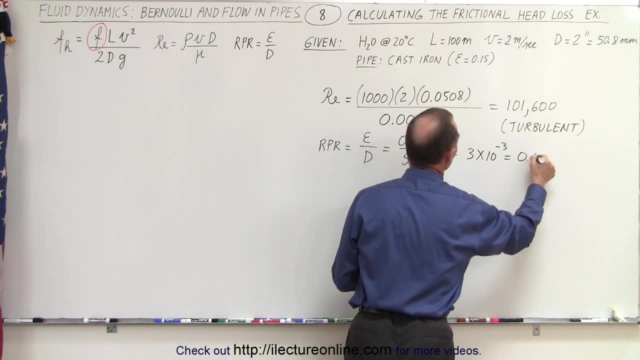 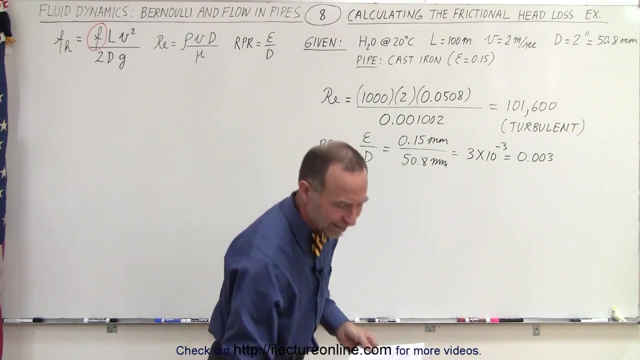 divided by 50.8, that gives us 2.95, or let's say three times 10 to the minus three is equal to 0.003.. Now, of course, we need a Moody diagram, and I happen to have one right here, just handy. 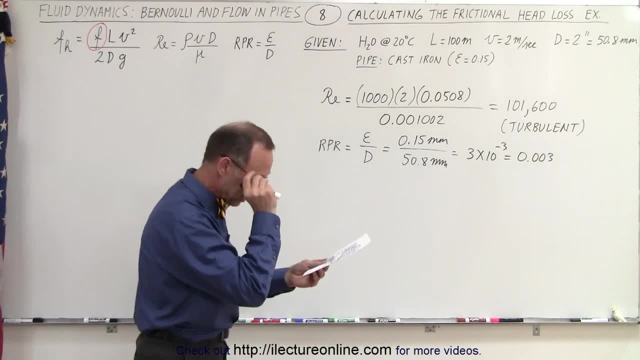 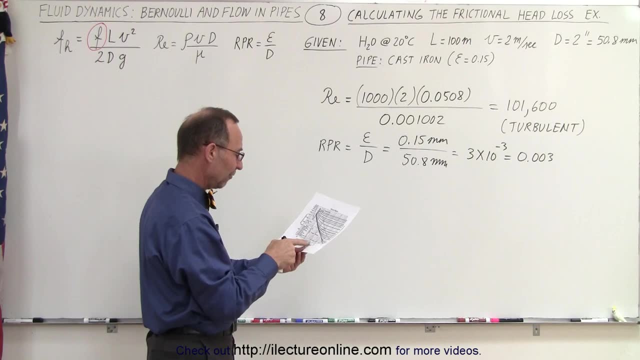 And, of course, to see the little details, I'm going to need to put on my reading glasses to see what we're doing here. So first of all we go to 101,600.. So that's basically 10 to the fifth. I find a point on the Moody diagram that says 10 to the fifth. 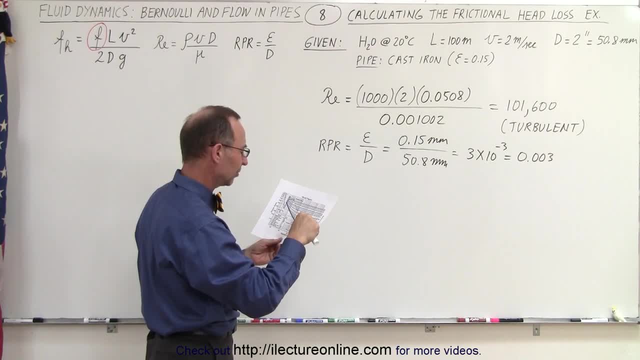 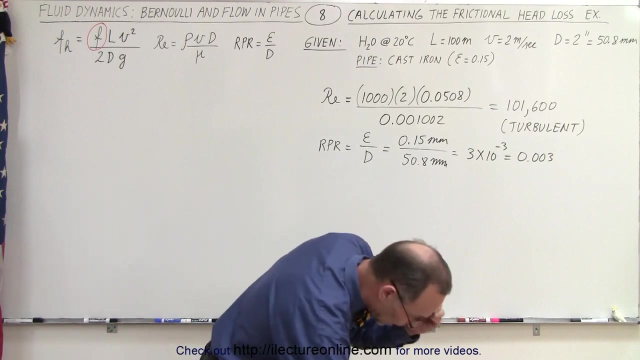 And then I find a relative roughness of 0.03- that's somewhere between 0.02 and 0.05 right here. And then I go across here And I find that I have a friction factor of approximately 0.028.. 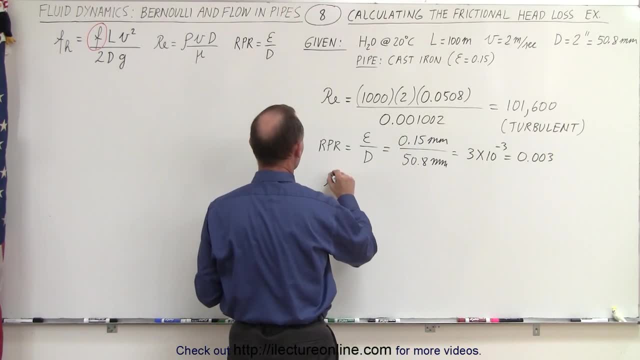 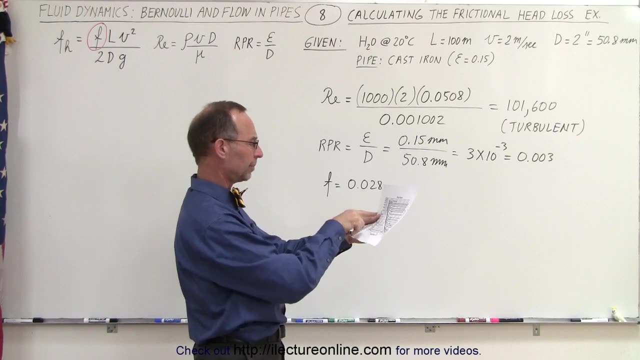 All right. So that means, from using this, that the friction factor is equal to 0.028.. And let me quickly check that again: 0.03,, 0.02,, 0.038.. Yeah, that's probably a fairly good estimate, All right. Again, it's approximately. 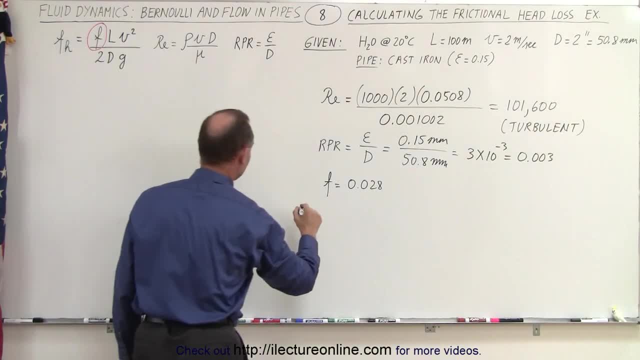 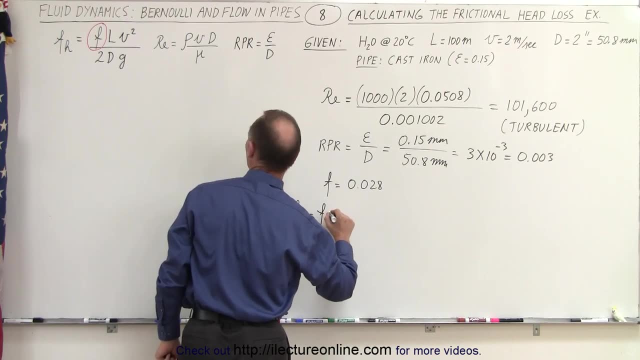 So now that we have the friction factor, now we can go ahead and calculate the head loss. So the friction factor, So right here, let's go ahead and put in the equation: F times the length, times v, squared divided by two times the diameter, times g. 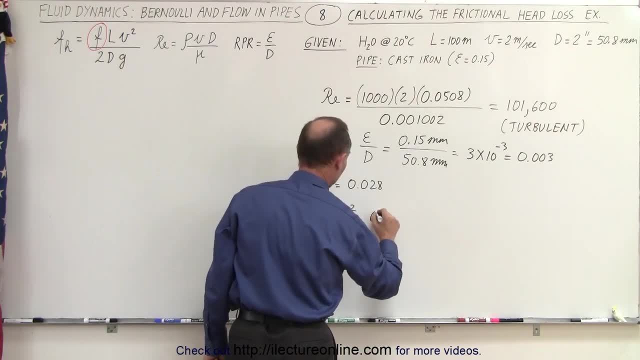 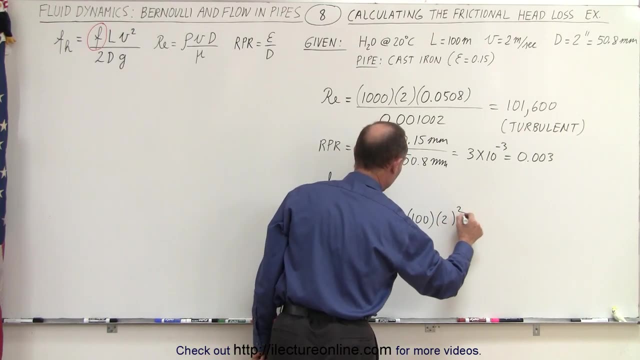 And of course that's going to be in meters. So we put on the factor 0.028 times the length, I had 100 meters, The velocity squared, which is two squared divided by two times the diameter In meters, which is 0.0508, and g, which is 9.8.. 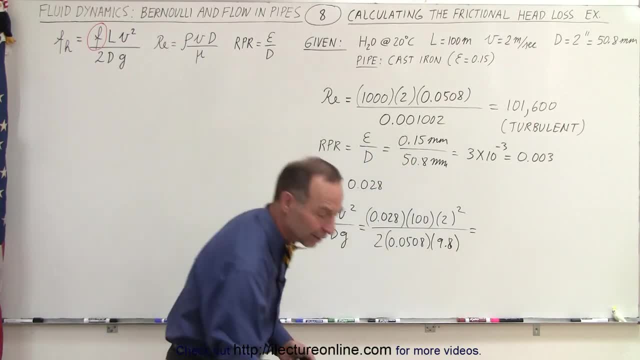 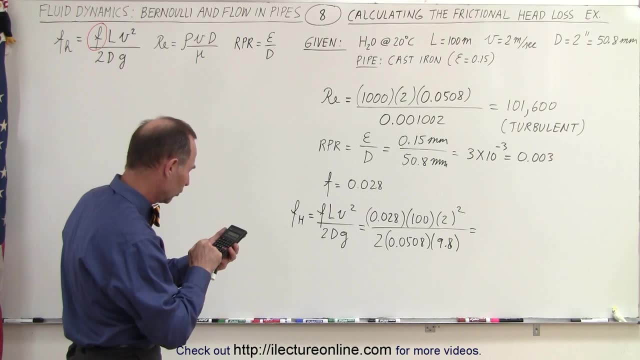 It's an eight right there. All right, Let's see what kind of friction head loss we're going to find. So 0.028 times 100 times 4, divided by 2, divided by 0.0508 and divided by 9.8 equals. 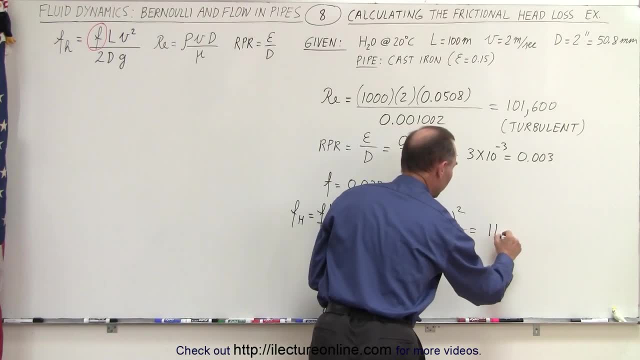 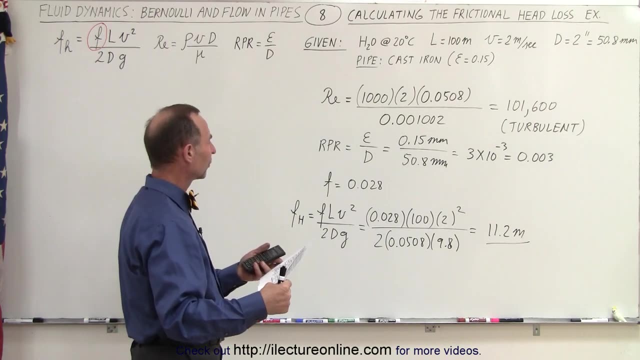 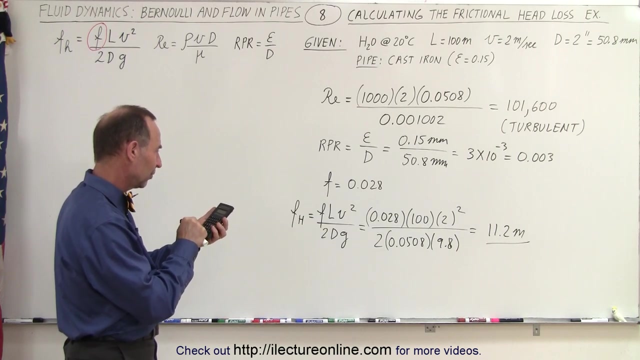 Let's end up with 11.8.. 11.2, 11.2 and that would be meters. Let me do a quick check again on the graph: 0.03, that looks about right. So we have: 0.028 times 100 times 2, divided by 0.0508, divided by 9.8, equals 11.2 plus 11.25.. 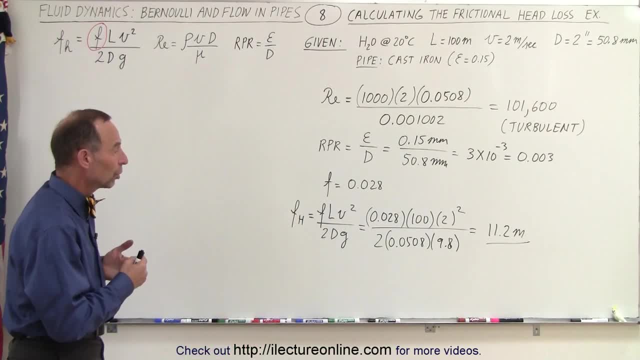 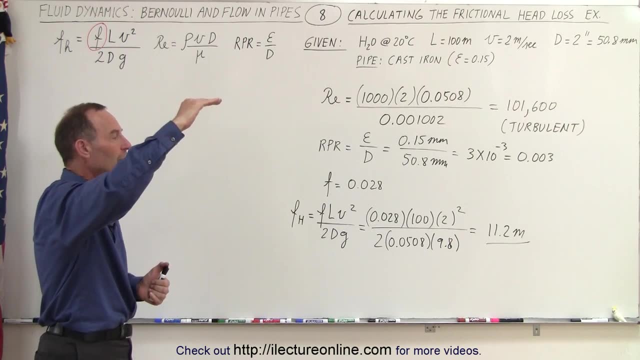 Yep, That's the frictional head loss. With other words, The equivalent is That it looks like we need to put in additional work, additional effort, as if we were to lift the water an additional 11.2 meters over a length of the pipe of 100 meters. 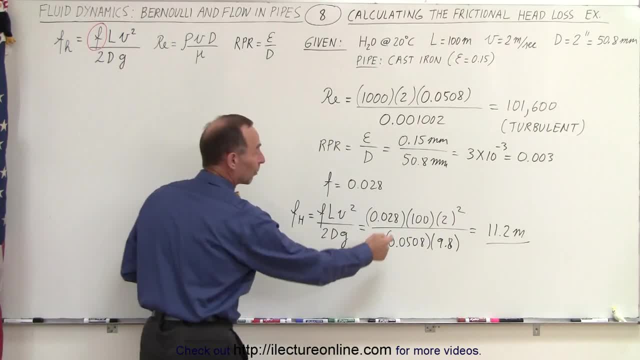 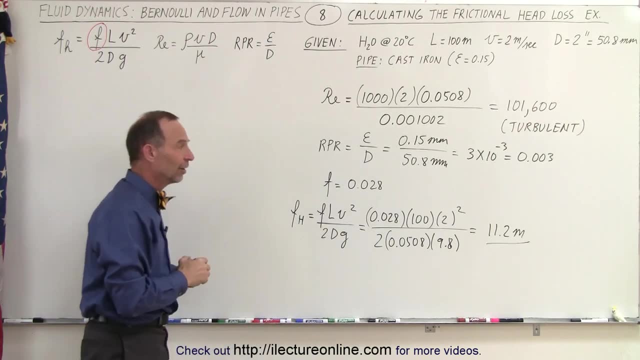 Part of that, of course, is that we have a very high velocity, The pipe is fairly long and we have a pipe that has a relatively high internal roughness of 0.15.. All that together with a small pipe diameter of only two inches. 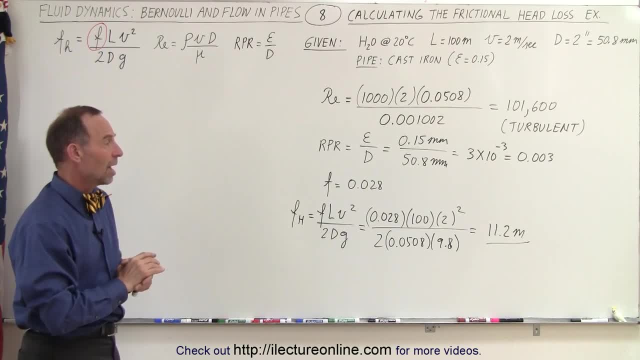 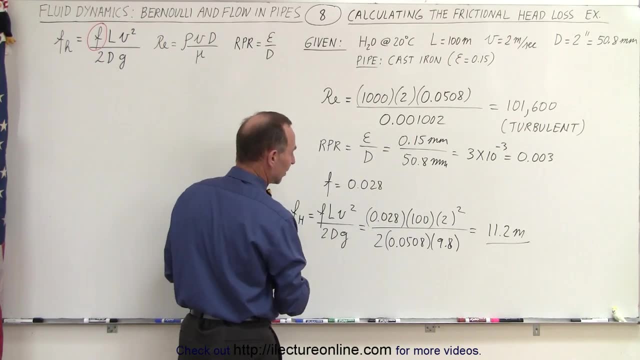 It's going to take a lot of effort to push the water through at that speed. How can we remedy that? Well, obviously, by making this into a bigger diameter and maybe using a different kind of pipe and maybe therefore not requiring such a high velocity for the throughput of. 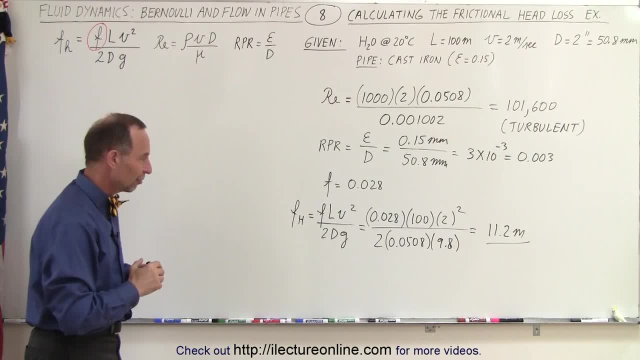 the volume of water and all that would definitely remedy that frictional head loss. So that's the kind of the way we want to look at it and that is how it's done.